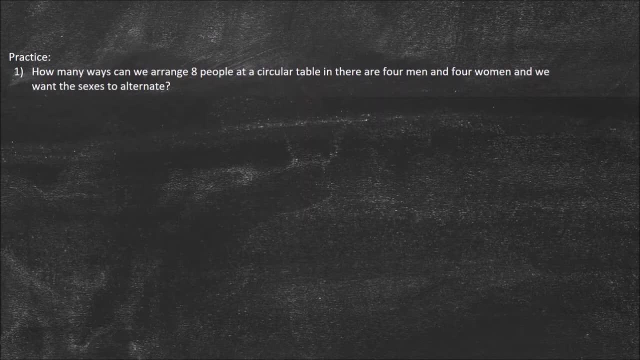 and we want the sexes to alternate Alright. so this is a tough one. So we did touch on this example in the last one, when we thought about how many different ways can we organize eight people at a table. but now there's a new constraint. 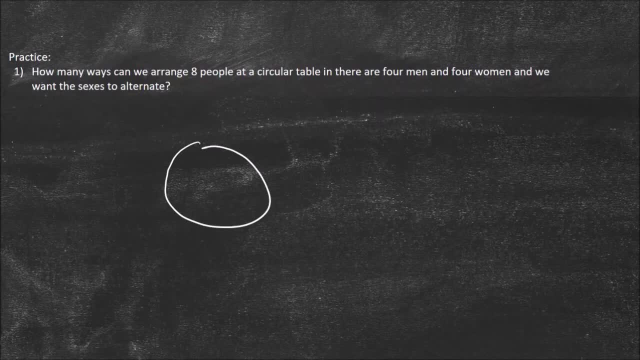 Because now there's four men and four women and they always need to alternate. So I'm going to draw my picture. It's going to be male, female, men, woman, men, woman, men, woman. Is that enough? One, two, three, four, five. 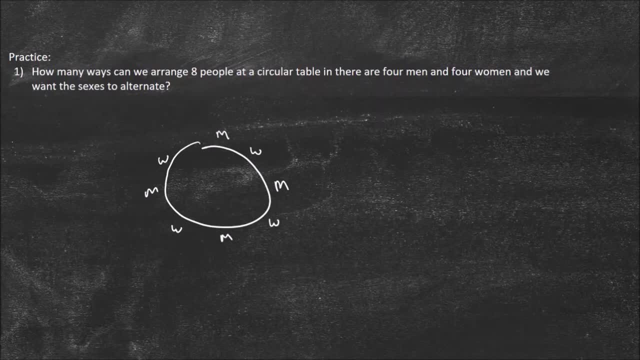 One, two, three, four, five, six, seven, eight. Okay, so we're good. So that's what it looks like When I do this. there's got to be eight people, but there's four men and four women. 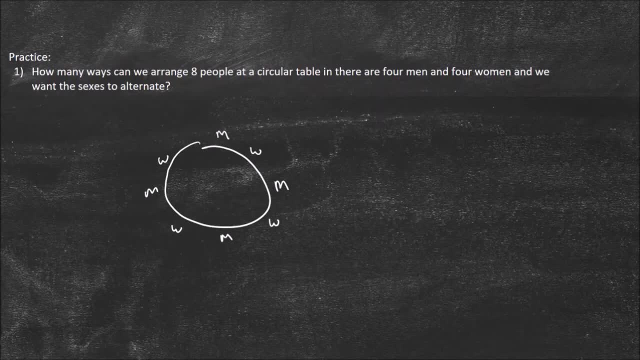 I'm going to kind of break it into two groups. How many ways can I organize the men? Well, there's four factorial right And we said again it's a circular table. So if I have four factorial ways to organize the men, but if I move all the men over one seat more, 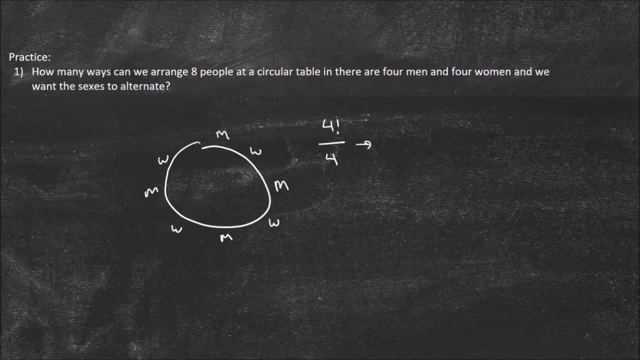 that would be the same thing. So I'm going to divide by four and that gives me three factorial. I just so you know that the reason this cancels to three factorial is that four factorial is four times three times two times one. divided by four, Those cancel and then we're left with three. 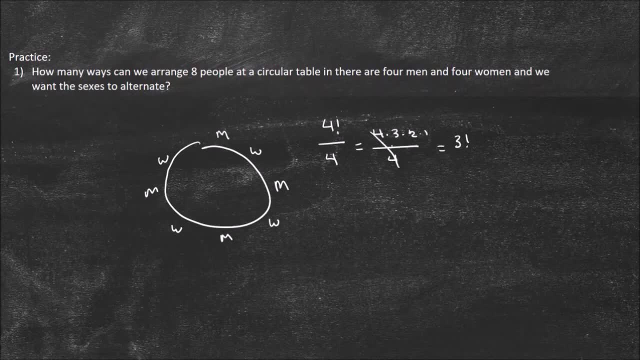 factorial, because that's three times, two times one. Okay, and then now, so this is the men, So this is the ways to organize the men. And now I need to multiply that by the ways I can organize the women, And I know the logical thing is to say: well, the women can be organized the exact same number of ways as the men. 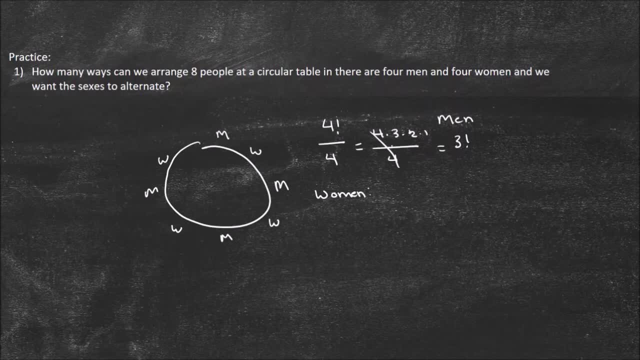 So three factorial times three factorial and we're done. Not quite, Because what we've done with the men is we've already accounted for the shift. This is um, this is for shifting the people, shifting people, So we can't account for that again. 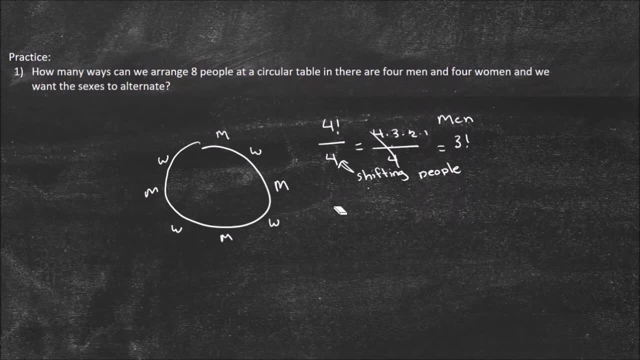 Now, the ways I can organize the women are going to just be the four factorial, because I can move them however I want, but it and if then, if I can move the men, the six ways, the three factorial ways, that'll be a new arrangement every time. So the women, the ways I can organize them, would be four factorial. 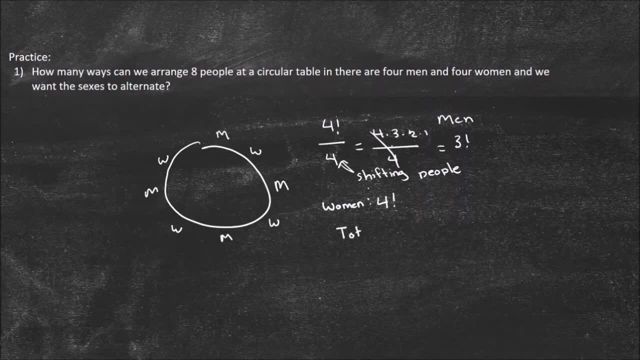 I would multiply the two together and my total would be three factorial times four factorial, and that would be the answer to my problem here. And what would that equal? Three factorial is six times four. factorial is four times four. 3 is 12 times 2 is 24, 6 times 24: 144. I think that's right. okay, you can check my. 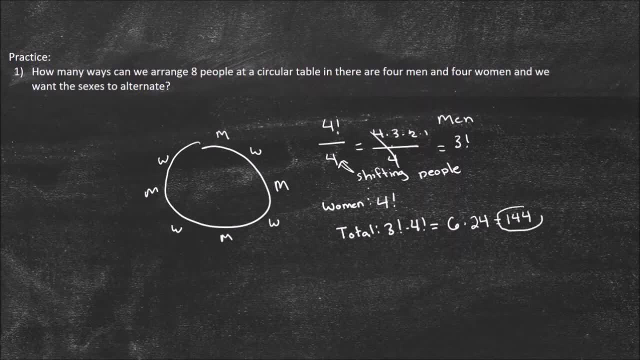 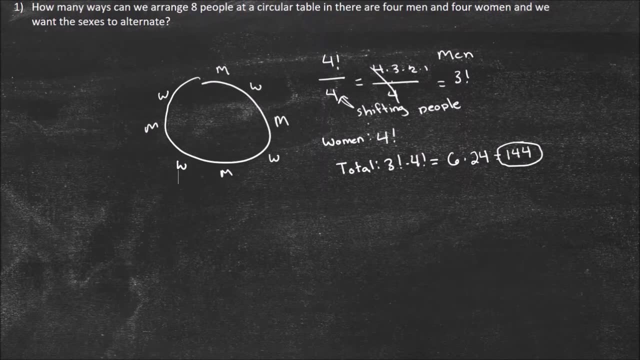 math there. all right, so 144 ways that I can organize the people at this table. another way to think about it is to say, okay, what if you, what if I? really liked that it was 4 factorial times, 4 factorial. I'm gonna write this one on. 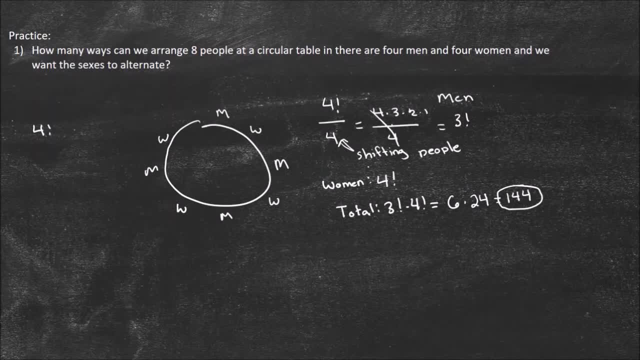 the left hand side. so I agree that it was 4 factorial for the men and then 4 factorial ways to organize the woman, and I just don't understand why we divided 4 only for the men, because that can be confusing one way I would like to. 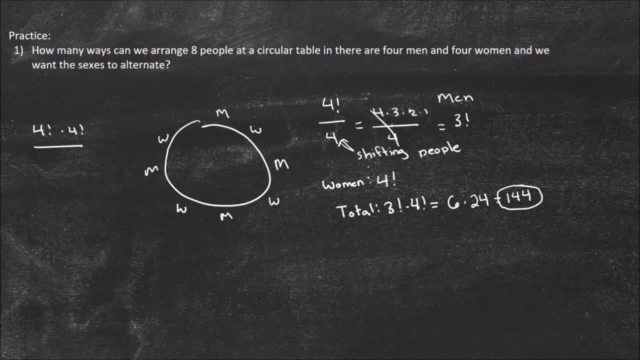 think about it is okay. so I did 4 factorial because that's the ways I could organize the males. I did 4 factorial. that's the way that I could organize the females. but then again, now we need to account for the fact that it's a 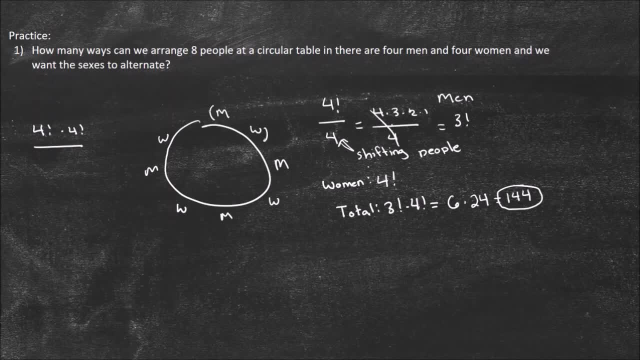 circular table. what I want to do is I want to, if I want, if male and female always have to alternate seats, well, we can view them as kind of a pair, so everyone's gonna be together. and if I moved all of this, if I moved both, all pairs, over one, I basically get a new table with pair one pair, two pair. 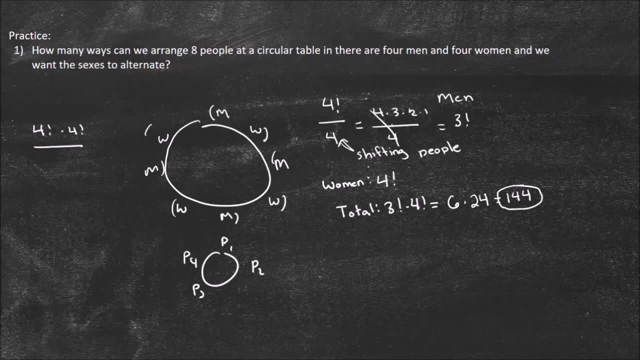 three and pair four, and I could move them all over one and it'd be the exact same arrangement: everyone be seated to this, next to the same person. the sexes would still alternate, but it's a circular table, so it's actually the exact same thing. so that gives me divided by four, which would give me the 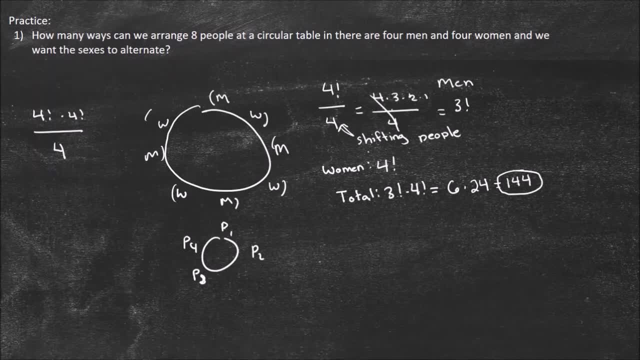 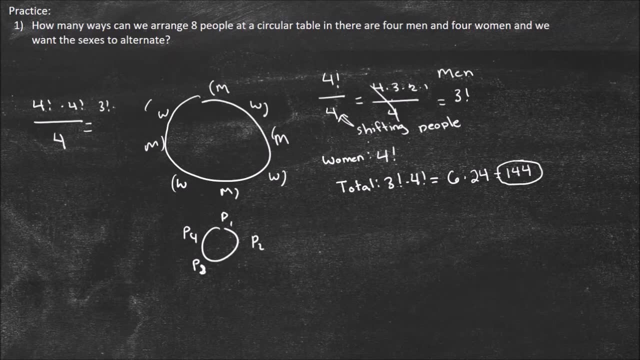 same answer as I had before. so if that really didn't make sense, why we only accounted for the shifting with the males? hopefully this what can offer you another way? and because this would simplify to three factorial times four factorial divided by four again, oh well, it would just be three. 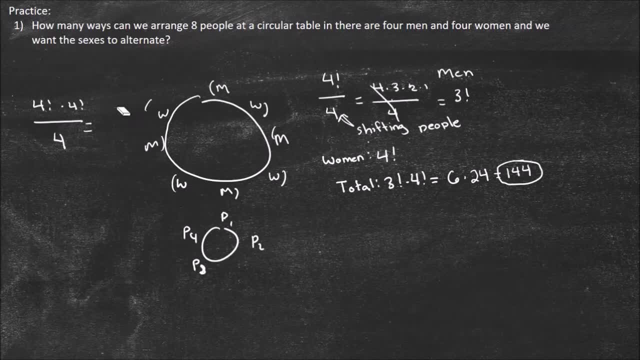 factorial divided by four factorial, because of the fours would have cancelled out from one of the four factorial, so that equals three factorial times four factorial, which again is the same 144. so that's just another option for you if this kind of was confusing. this is a tough problem though, so let's. 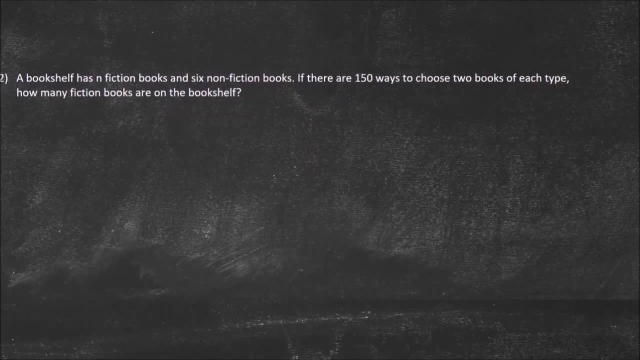 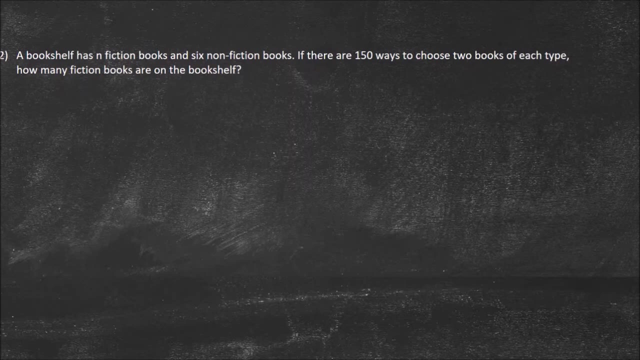 go on to the next one. all right, so now a bookshelf has in fiction books and six nonfiction books. if there are 150 ways to choose two books of each type, how many fiction books are on the bookshelf? okay, so I've got a bookshelf that has some fiction books. it's got. 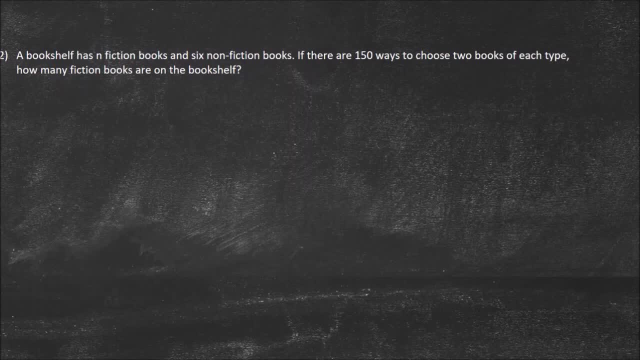 some non-fiction books. I'm trying to take two fiction books and two nonfiction books. I need to figure out how many ways can I do that. so I would. is this a permutation or combination? well, it's going to be a combination, right, because if I have the same, 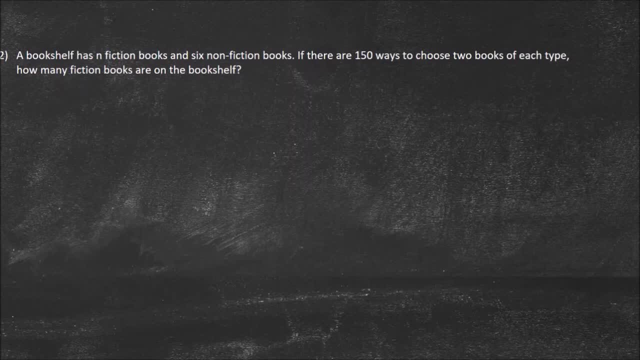 group of books, it doesn't matter which order they're in. So if I took Harry Potter and then I took I don't even know a non-fiction book, If I took them but then I took the non-fiction book and then the Harry Potter book, it would be the same thing. There's no concept of order here. 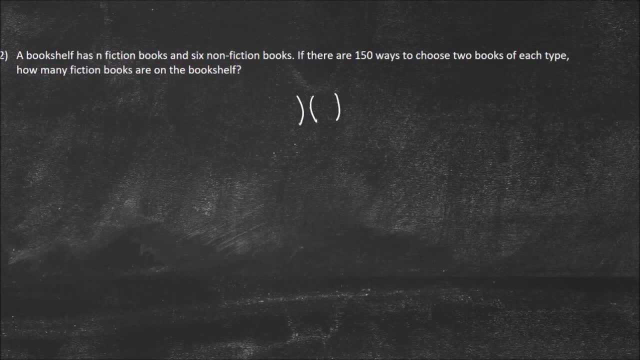 So it's going to be two combinations here and they're going to be multiplied by each other, right? Because this one's going to be the fiction. There's going to be a fiction combination and there's going to be a non-fiction combination. We're going to multiply them together to get the 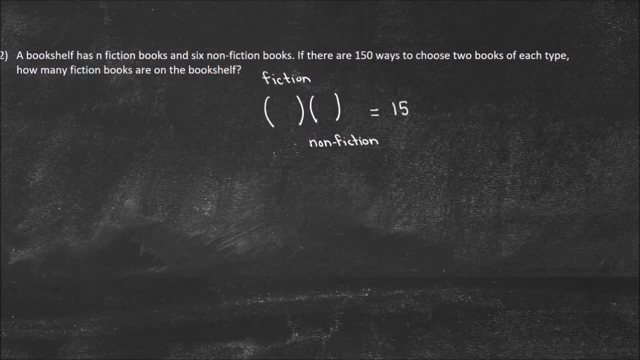 total combinations that I have, And I know that the total combinations that I have is 150.. There's 150 different ways And I'm actually given all the information about the non-fiction books, right, I have six and I'm choosing two of them, right? So six, choose two. 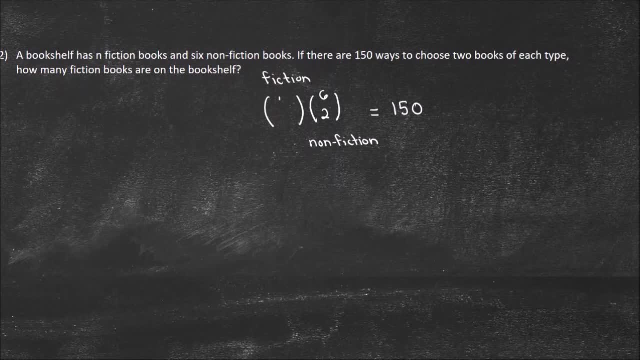 And now for fiction, I have n of them and I'm choosing two again because I'm choosing two books of each type. So this is the formula that I have, and now I just need to use my formulas to figure this out. So the 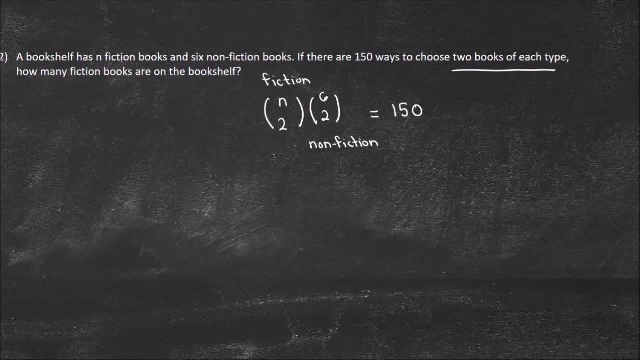 the key here was recognizing that this is a combination. then now you need to use the formula for combination and remember that n choose r equals n factorial divided by n minus r factorial, times r factorial, and that's what we need to apply to this question. so first i'm going to 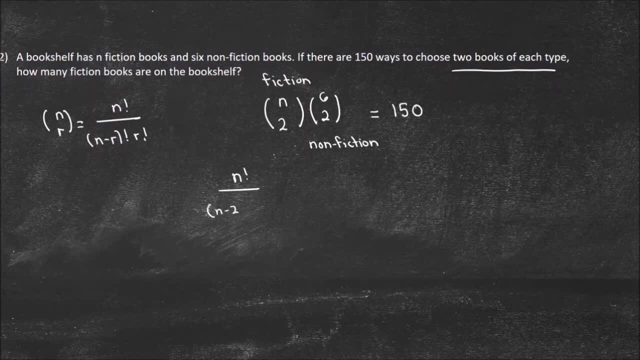 have n factorial divided by n minus 2 factorial times 2 factorial, because 2 is r multiplied by 6 factorial times 6 minus 2 factorial times 2 factorial. i'm going to simplify that up a little bit. so n factorial divided by n minus 2 factorial. well, n factorial is n times n minus 1 times n. 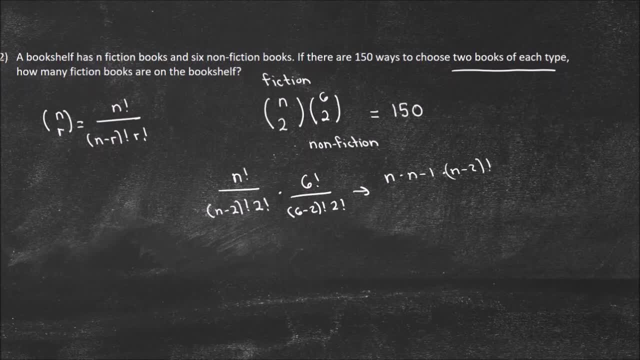 minus 2 factorial. that's just the definition of a factorial, so the n minus 2s are going to cancel out, so i'll write it here anyway, though. so that's going to be gone. then i'm left with 2 factorial multiplied by 6. 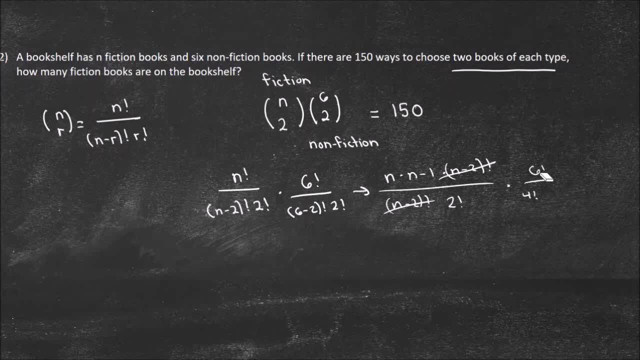 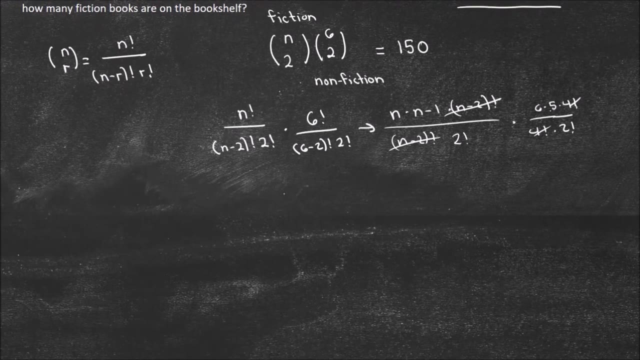 factorial divided by 4 factorial. if you notice, i can multiply out this 6 factorial into 6 times 5 times 4 factorial. the 4 factorials will be gone. times 2 factorial. so 4 factorial gone. and i'm going to simplify on the bottom here. i'm going to get be left on the top with n times n. 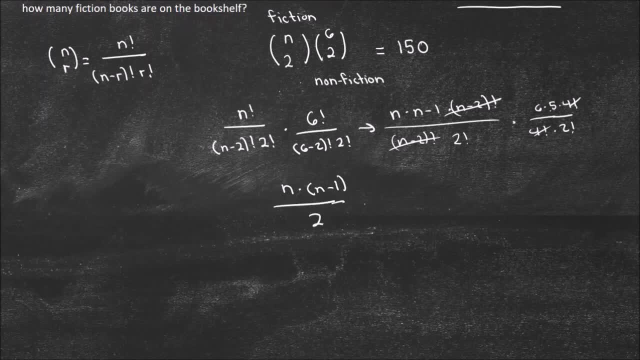 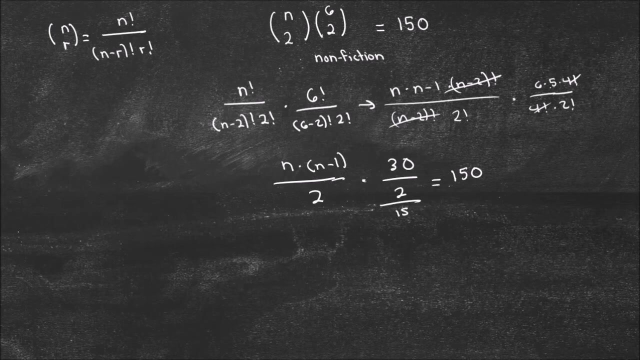 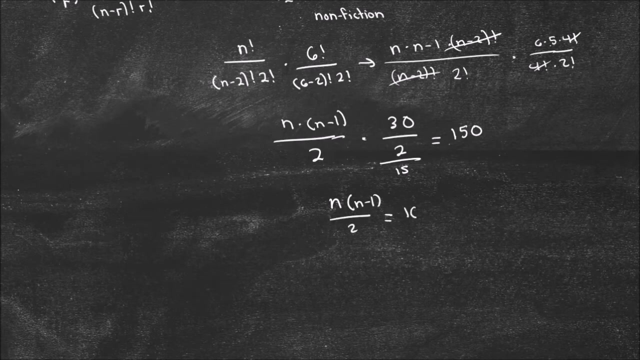 minus 1 divided by, instead of 2 factorial, i can just say: 2 multiplied by 6 times 5 is 30. divided by 2 factorial is 2, 77.. equals my 150.. 1aki times n minus 1 divided by 2 equals 10, because i divided 150 by 15. 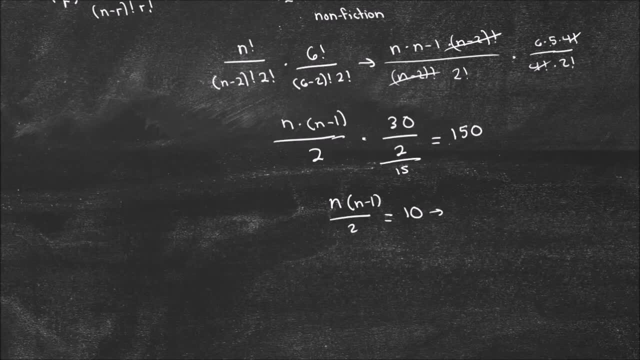 99.. and then now i do, i'm going to multiply by 2 and i'm gonna n times n minus one equals 20.. 2 pi, jazz 1, 5 pi. and now i just have to solve a little quadratic so i get n squared minus 1, specialized for our 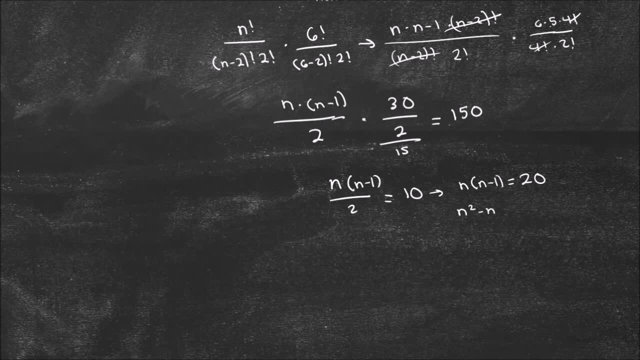 square со spin: 1, 25, 26, 0, 1, 76, 84, 99, 280, 52, lol. n equals 20 and I'm going to bring the 20 to the other side. get n squared. minus n minus 20 equals. 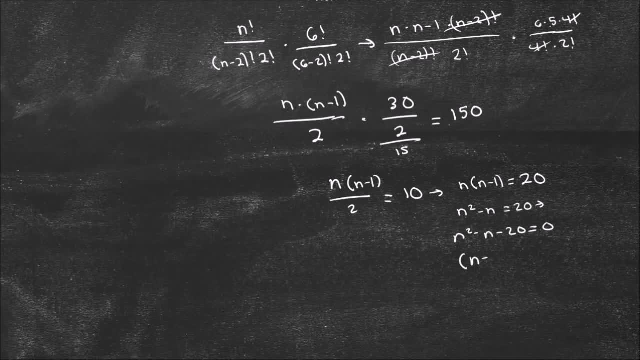 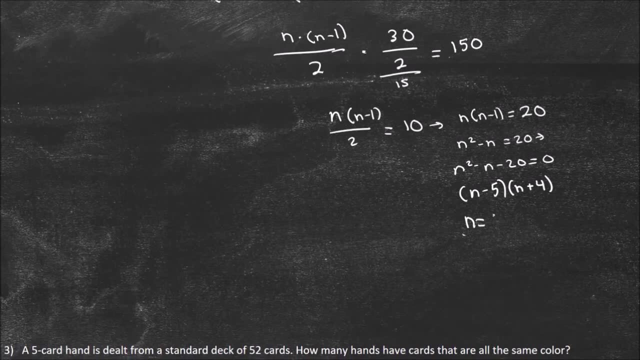 0, n minus 5, and then when I factor that out I get n minus 5, n plus 4. so officially n can equal 5 or negative 4, and logically, which one does it have to be 5, right, I can't have negative fiction. 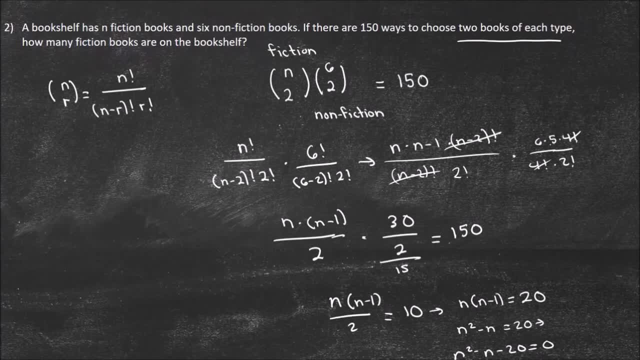 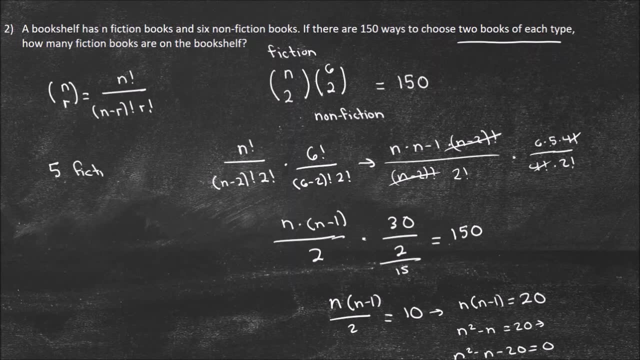 books, so n's got to be 5 and what that means in terms of the problem is how many fiction books are on the bookshelf. there's five fiction books, so hopefully that makes sense. hopefully that shows you kind of. this was a good problem to get you really thinking about combination formulas and 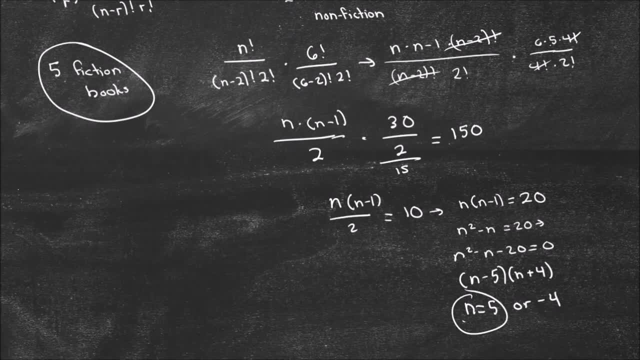 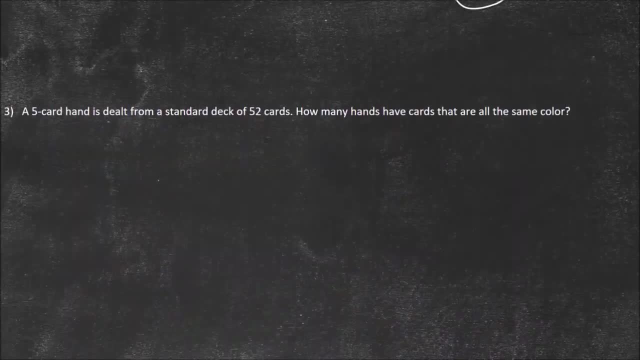 then also factorials. you really have to understand factorials to be able to recognize that all the cancellations that you can make here. so the answer is that you have five fiction books. hopefully that makes sense. all right, and we have one more here. this one's not too bad. a five card hand is dealt. 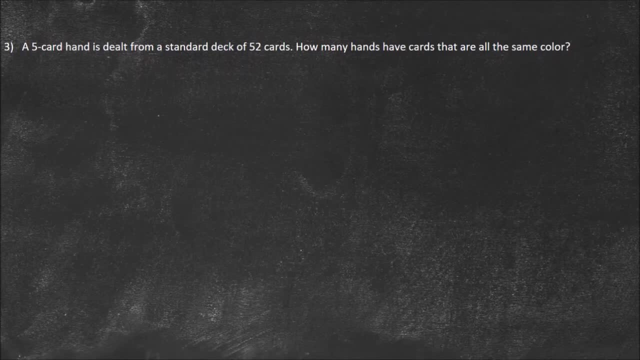 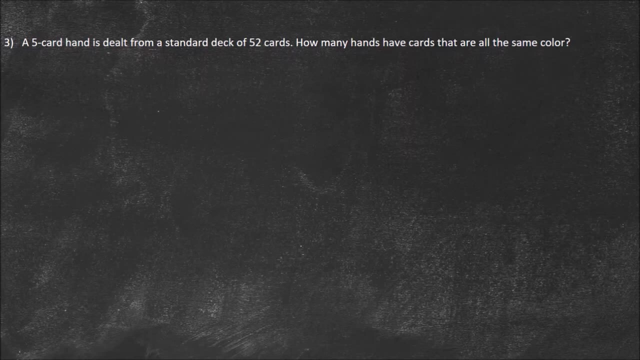 from a standard deck of 52 cards. how many hands have cards that are all the same color? so is this a permutation or a combination? well, it's going to be a combination, because if I have the exact same hand but I was giving them in a different order, it 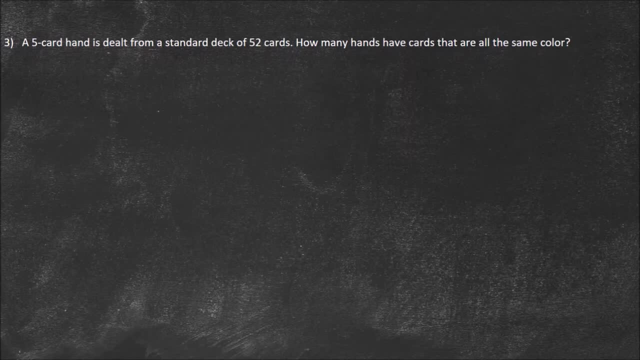 wouldn't matter, they would be the same hand. so that means it's not going to be a permutation, because with permutations order does matter. this time order doesn't matter so well, if I have. so, let's consider the color. so colors a standard deck of 52 cards. there's 26 that are red, my hearts and 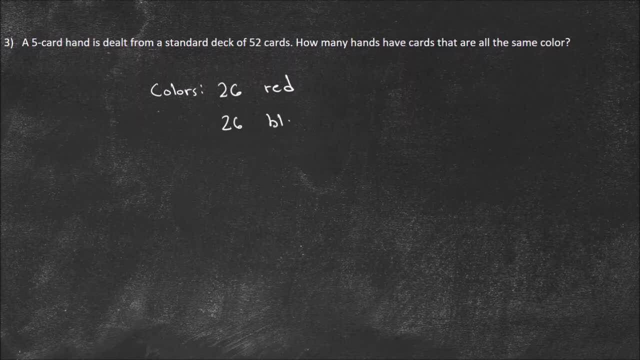 diamonds, and then there's 26 that are black: the clubs and spades. I want to know how many five card hands have cards that are all the same color. Well, first I'm going to think about my red hands. So red hands and the 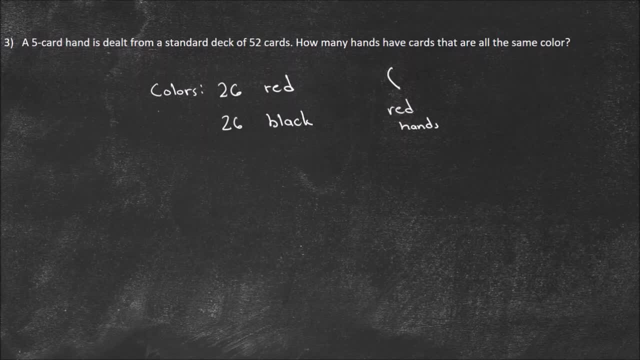 thing is you're going to notice quickly- you probably already know- is that the number of hands that are all red cards and the number of hands that are all black cards are going to be equivalent, and the formula is just going to be 26. choose 5, because there's 26 cards that I can. 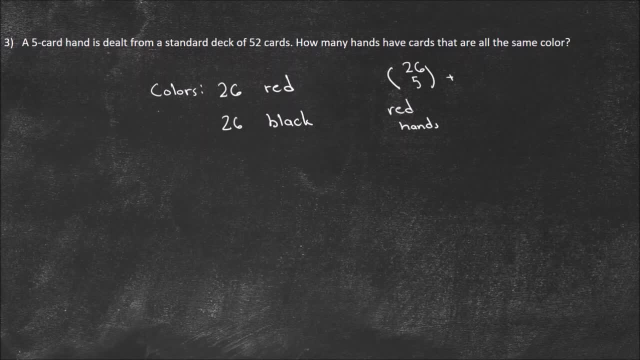 choose from, and I need to take a five of them and then plus. now for the black hands, it's also going to be 26 choose 5, and these are black cards. So this would be a hand of full black cards. So that's the answer. It's 26 choose 5, times 26 choose 5, or plus 26 choose 5. and if you wanted, 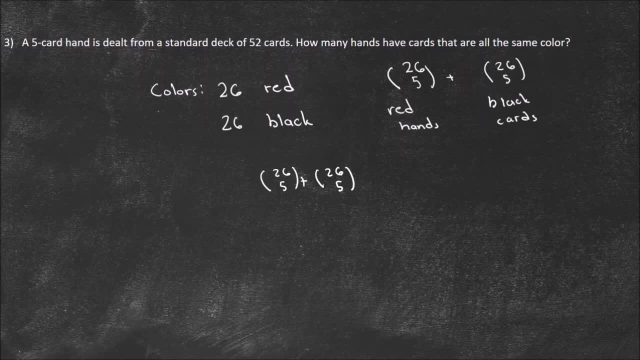 to simplify it you could. I would not recommend it, though It would be kind of. it would be a bit of a pain. So this would be the answer that most tests would accept: that that's the number of hands that would have cards that are all the same color. A common question is: what is the probability? So 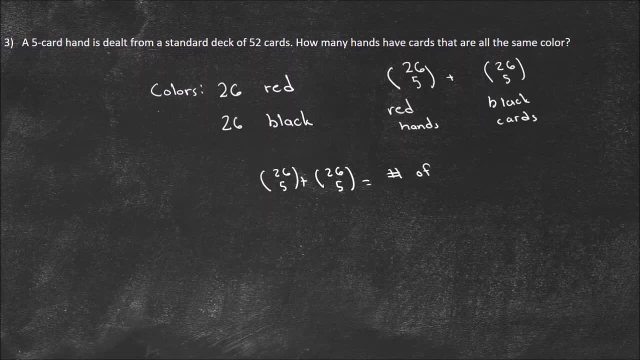 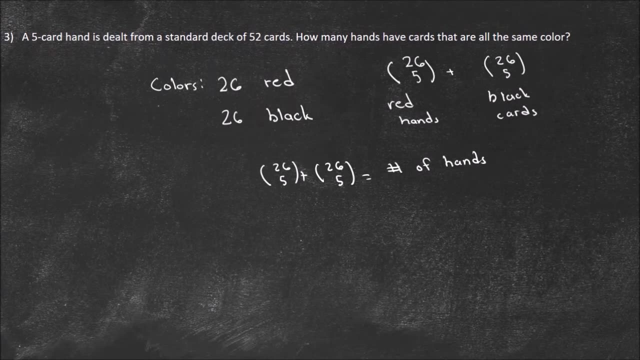 these. this is number of hands. number of hands. Okay, what about probability of drawing a hand that has cards of all the same color? And this is important for like poker or something? maybe you wanted to know this. Well, it'd be the number of hands that are all the same color: 26 choose.